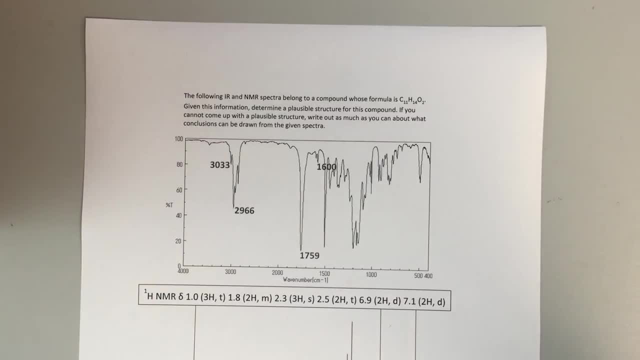 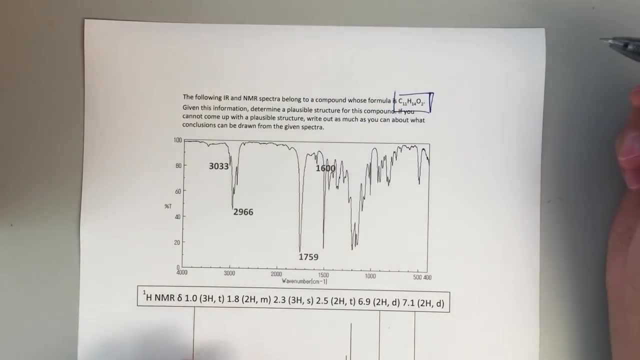 All right class. so this is sort of the big picture problem for our IR and NMR spectroscopy sections, And this problem is asking us to sort of come up with a plausible structure for a given molecule. The information that's given to us is the formula. So we've got C11H1402.. 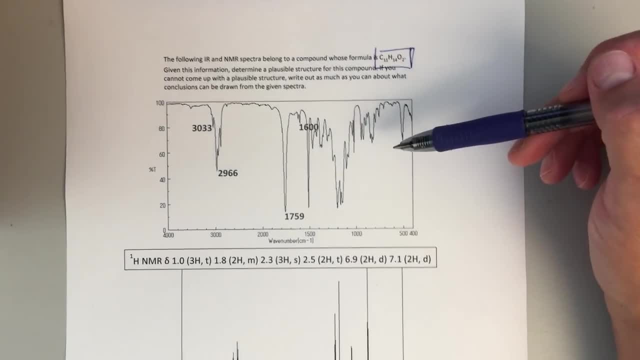 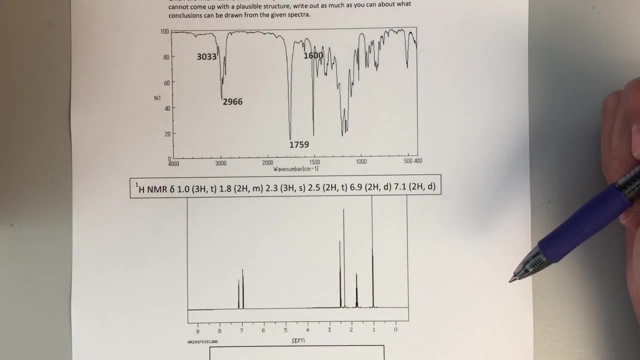 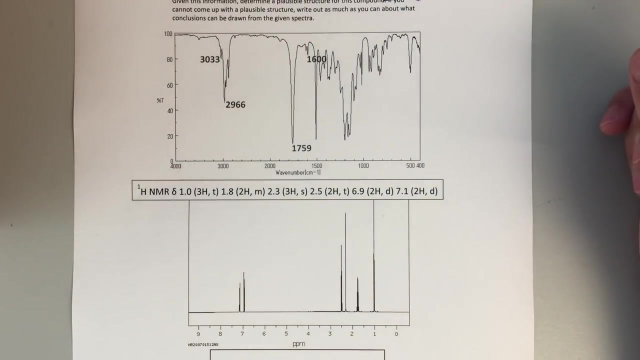 And we've got an IR spectrum with some peaks that are labeled and an NMR spectrum with all of the NMR relevant NMR data for us. So I'm going to talk through sort of the strategy behind you know a problem like this, how I'd like you guys to sort of write everything out. 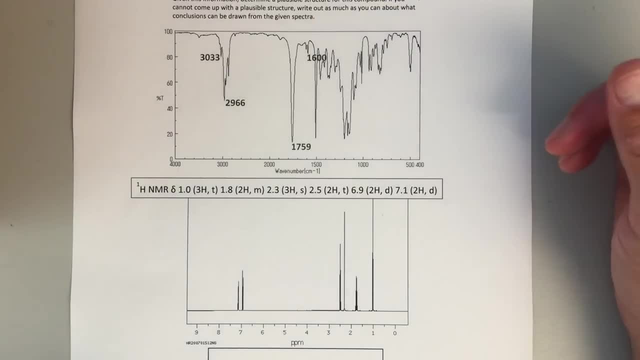 and then how we can sort of come to a plausible structure for you know a final product and then check to make sure that everything sort of makes sense, that we're, you know, proposing something that is consistent with the data. That's the goal here. Okay, so let's get started. 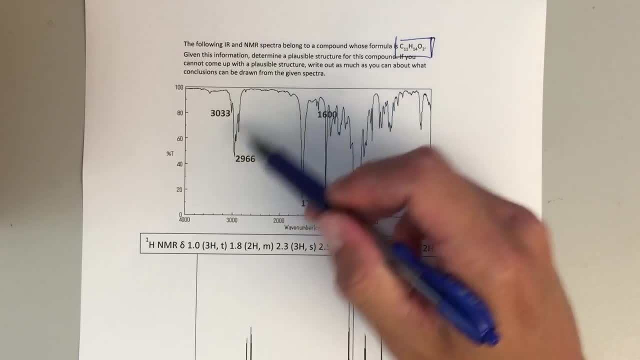 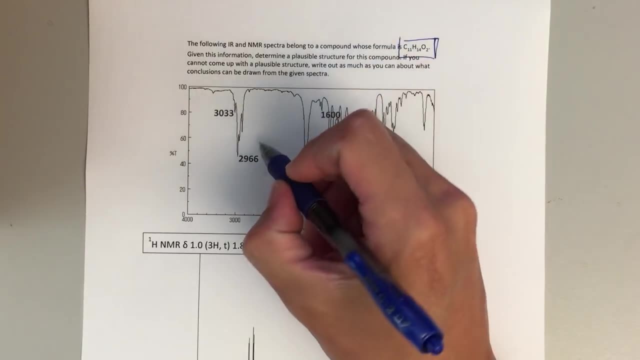 So the first thing that I would do is look at my IR spectrum and sort of label what you know, what I see Here. we've got some peaks just below 3000.. So right away I'm going to say SP3CH. So 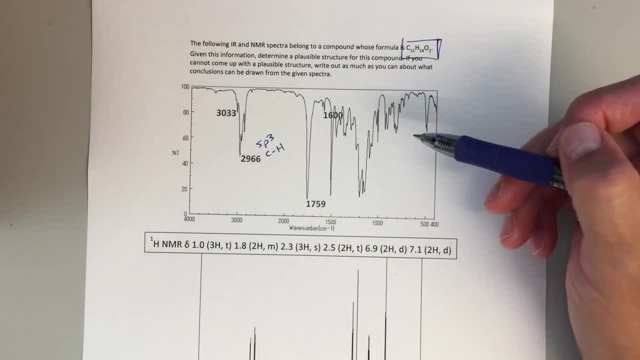 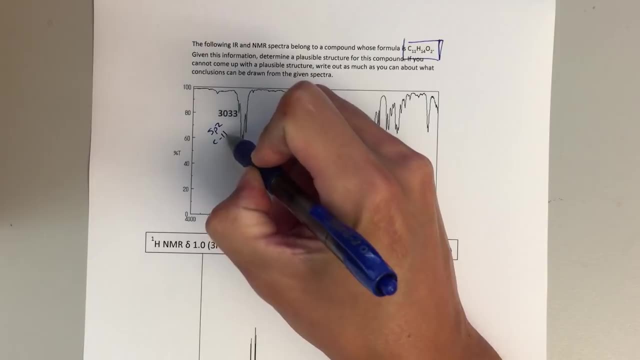 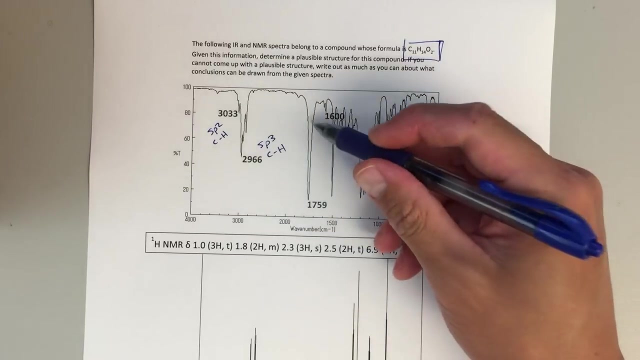 we've got some, you know, alkane type SP3CH bonds that are stretching there, This 3033, that's going to be an SP2. CH so just above 3000.. That's my SP2 hybridized CH bonds At 1759, so I think that this is pretty. 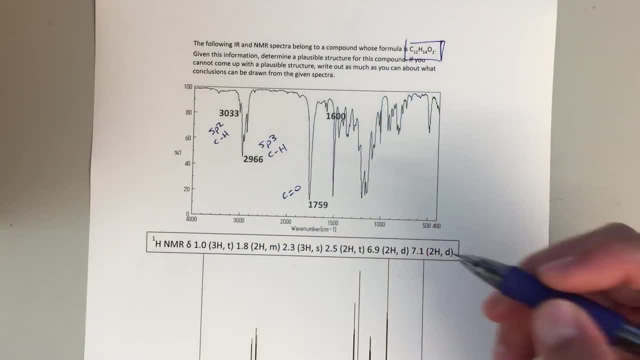 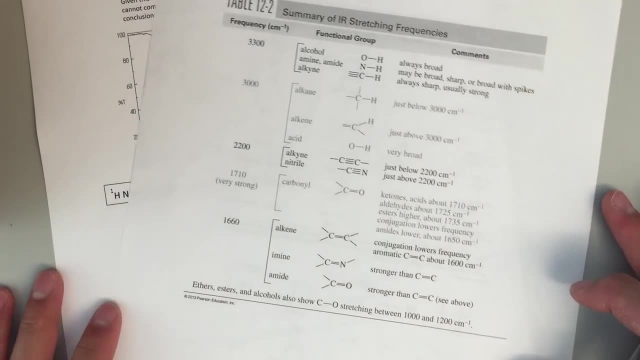 clearly a C double bond O, And then we can sort of think about: well, what type of C double bond O, what type of carbonyl stretch is that? So if we go to our table here, here is our, you know. 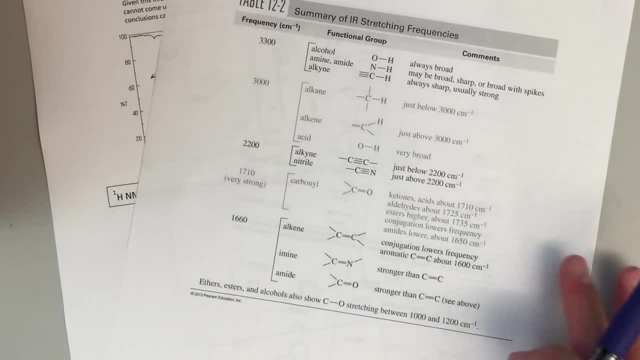 C double bond O. We've got ketones acids about 1710.. So again we're at 1760 pretty much. We also have a C double bond O which is about 1710.. So again we're at 1760 pretty much. 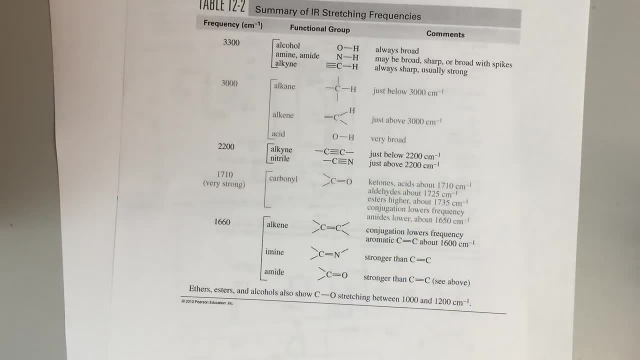 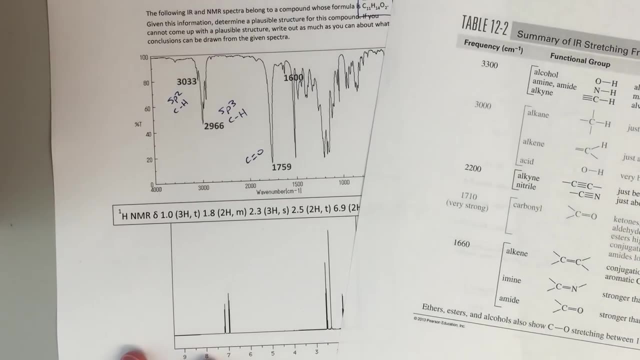 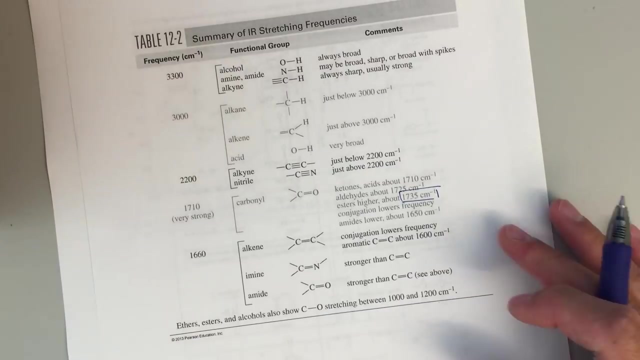 That conjugation is going to lower the frequency. So probably not a ketone or acid Aldehyde. 1725.. Again, we're sort of you know this is a little bit higher than those numbers. Esters, that's the highest one we have here, So about 1735.. So I might be thinking ester here. 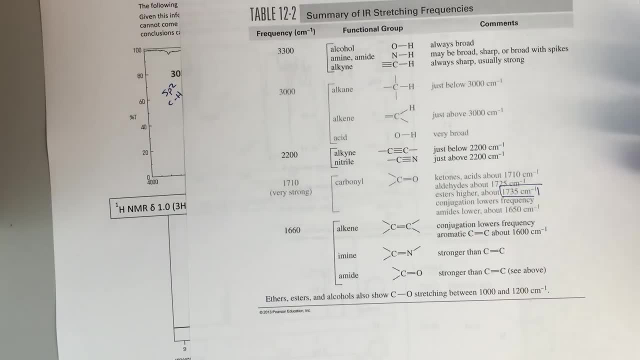 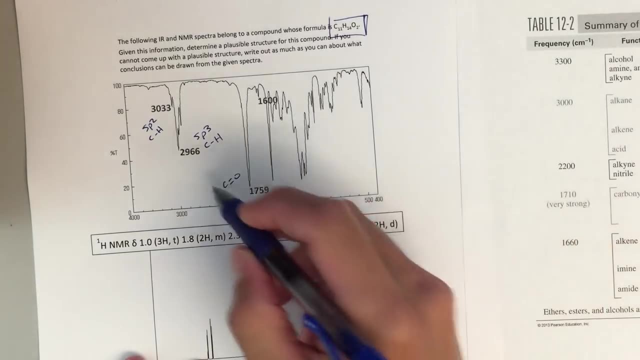 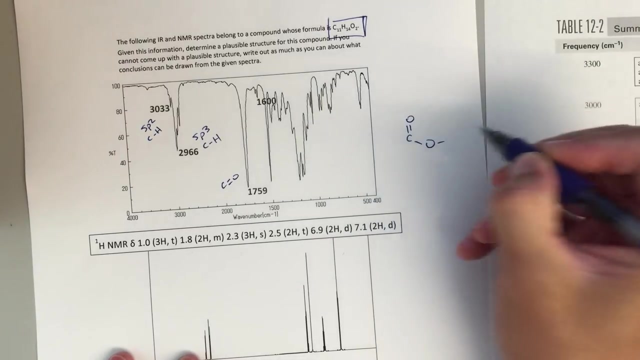 you know, looking at what else you know fits, That's really the only thing I'm sort of finding on here, So that's going to be my guess at this point in time. So for this C double bond O, I'm going to guess you know something like this with some other. 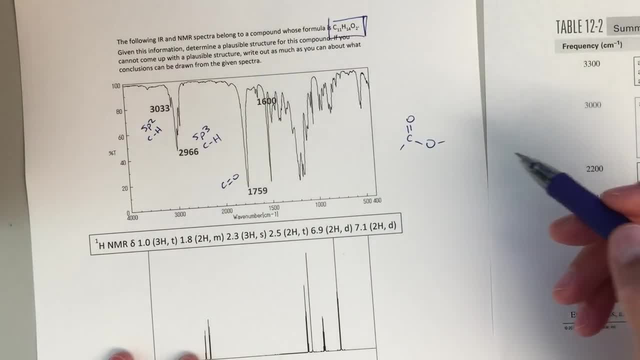 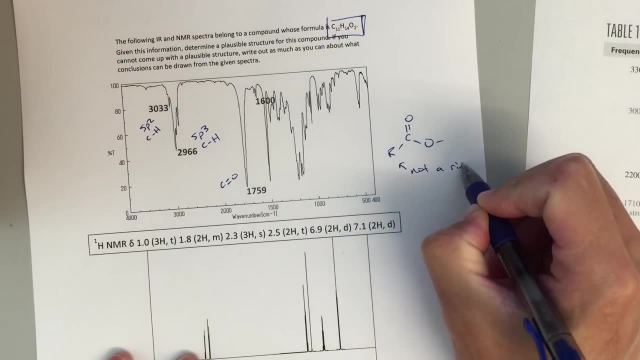 stuff going on here. So I've got a generic ester here. I'm going to put an R group here and I'm going to say not a ring, And I'm going to say that that's not a ring on this other side of. 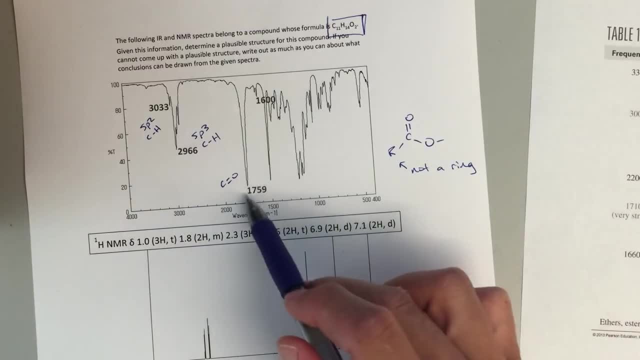 this, you know, carbonyl stretch, because this is so high It doesn't. if it was uh conjugated, then that stretch would be lowered. It would be, you know, I would expect it to be below 1735.. But since it's above um, I'm going to say definitely, we don't have conjugation going. 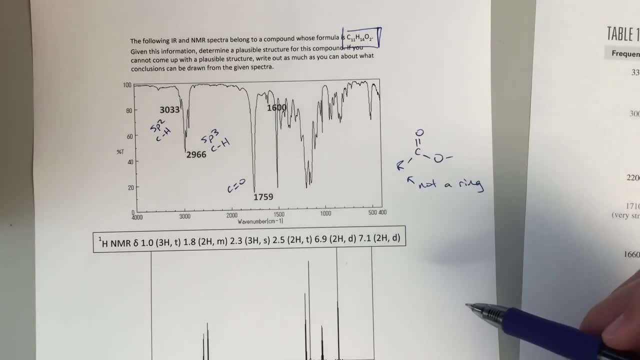 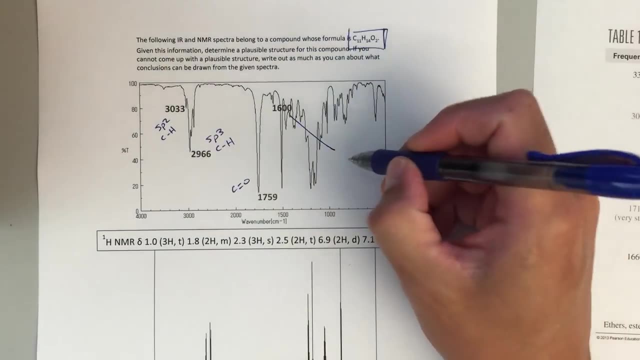 on here. So I'm going to put not a ring um for my ester, But I think that's a good, you know a good- start. 1600, that is going to be a benzene ring right. So whenever we see 1600, we're going. 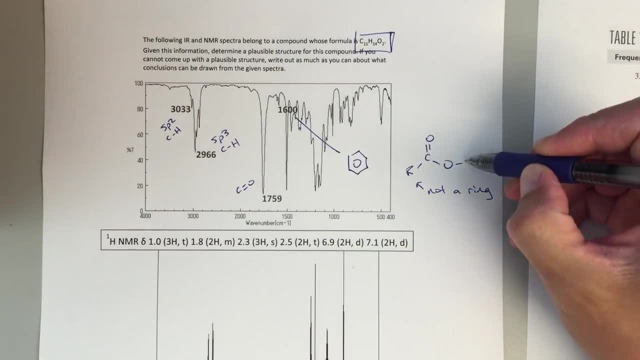 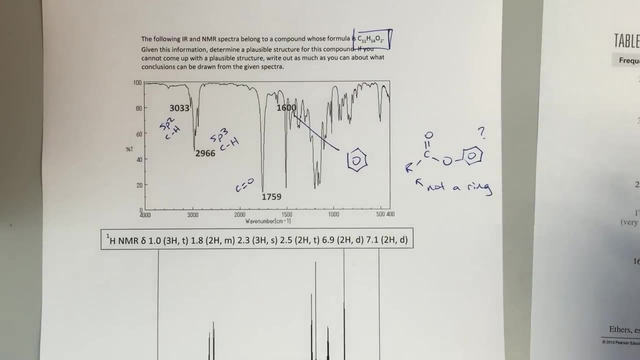 to think that that's a phenyl ring. So maybe that phenyl ring's over here, right? So we could say: well, you know, maybe we've got some ring over here, because there's clearly a ring in my structure, Um, but I don't. I know that it's. 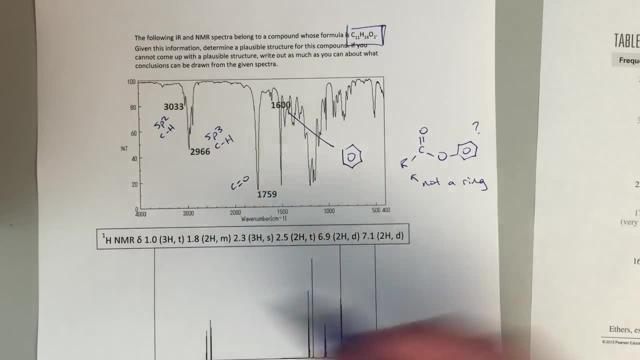 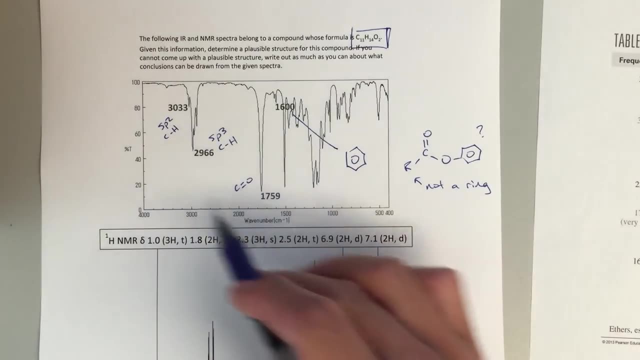 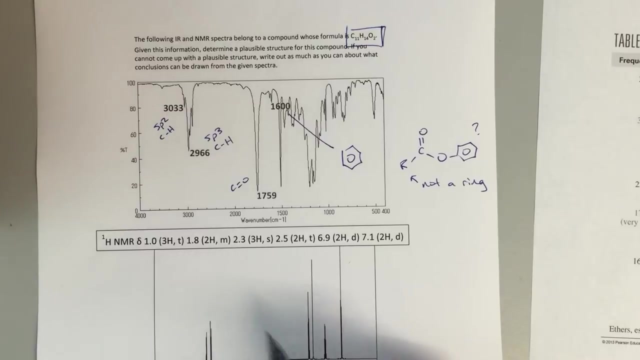 on this side, because this 1760, um would be much lower Conjugation would lower that frequency, uh to below 1735 for sure. So that's the conclusions that I can draw from my IR, And these labels I think are are very important, right? We need to have this sort of information. The sp2ch. 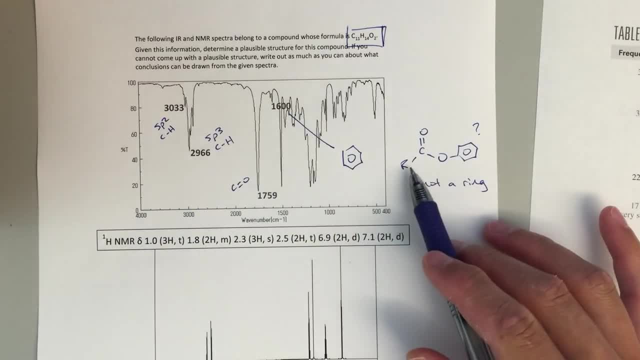 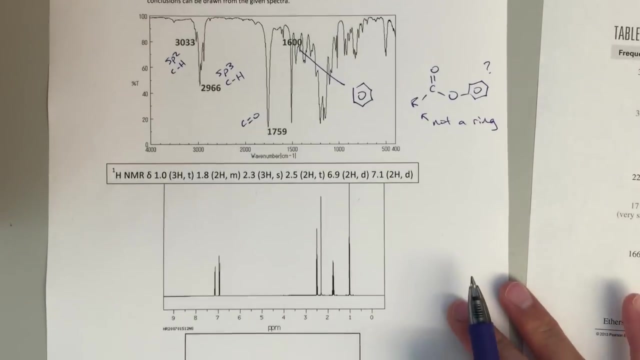 that can come from my ring So that that makes sense. This other R group that this sort of suggests that that's going to be some sort of R group. So that's going to be some sort of R group. So let's go to the NMR and see what we can find in the NMR. This is how I'm going to present the. 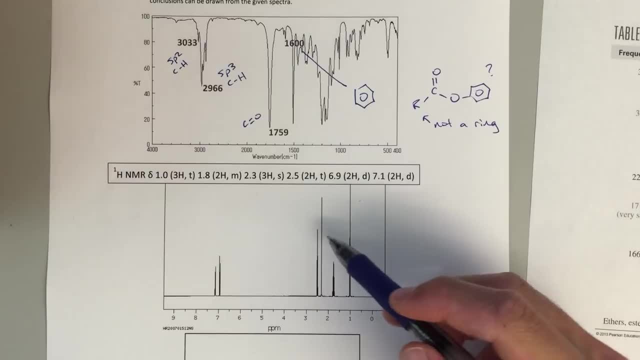 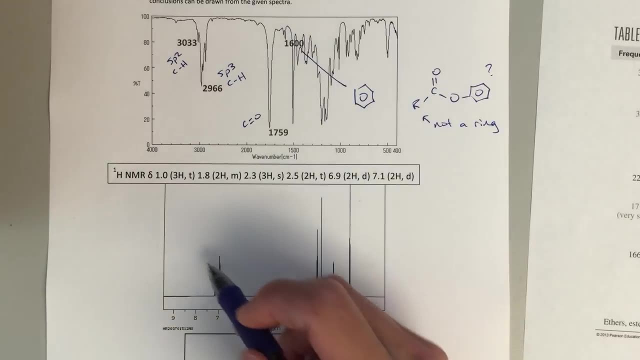 NMR to you And it's sort of hard to see. um, you know, it's sort of hard to interpret this. So what I would really recommend is labeling all these peaks. So out here, you know, I've got a too high. 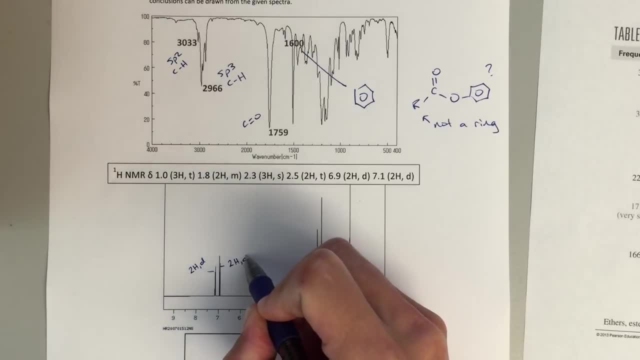 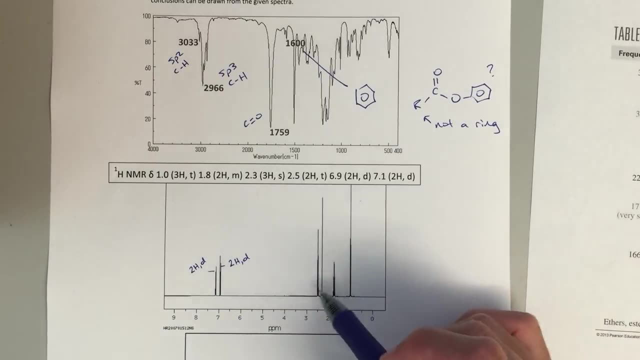 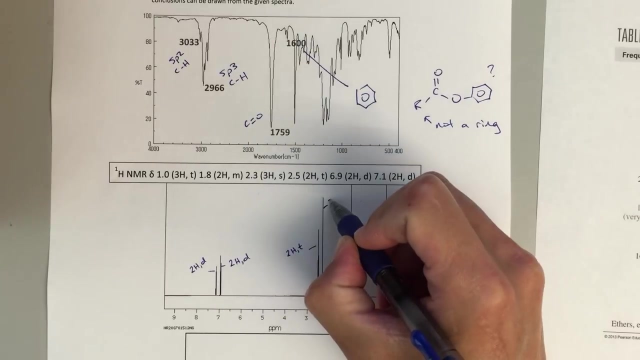 doublet. This one is again a too high doublet. So writing the information on you know the actual NMR spectrum makes it easier to interpret. So here at 2.5, this is a too high triplet. This peak, here at 2.3, is a three high singlet. So that singlet that's, you know right away. 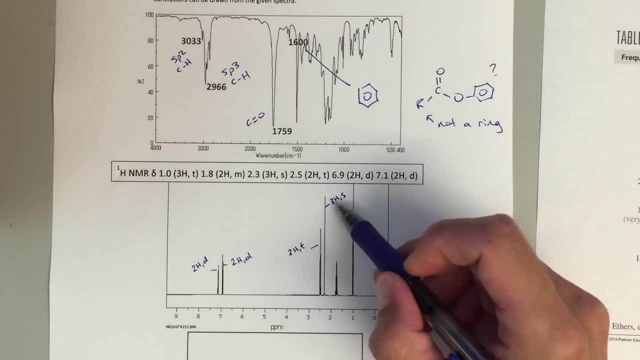 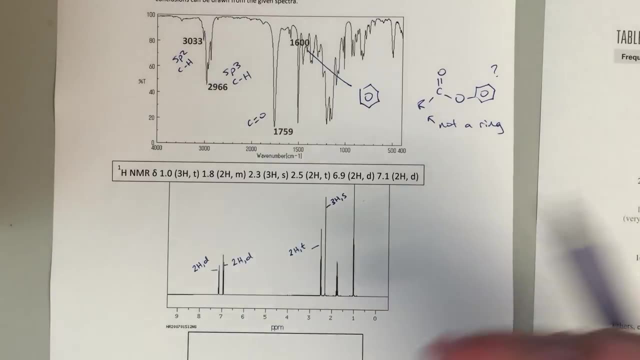 I'm sort of saying, oh, that's, that's pretty interesting. Um, there's a methyl group there, three high. it's probably a methyl group and it's isolated. Three high singlet means, you know, a methyl group that's isolated from other things. It's not part of an alkane chain Down here at 1.8,. 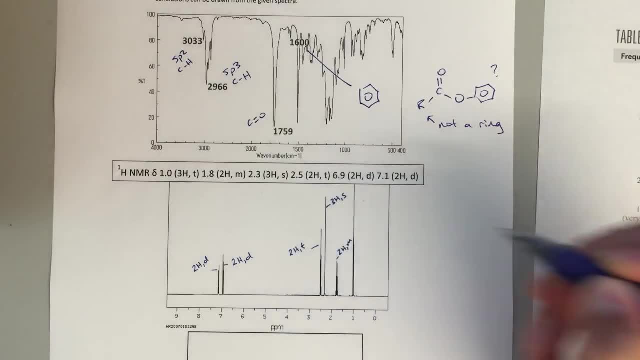 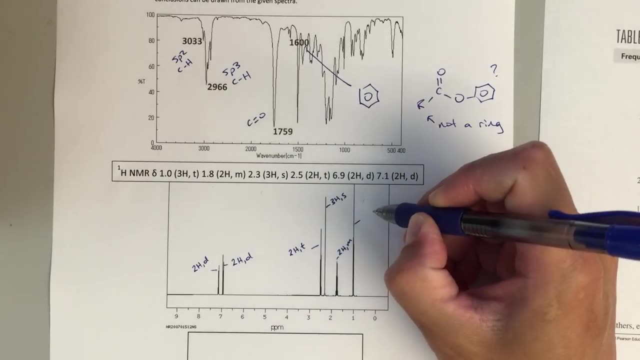 I've got a too high multiplet, Um, so M means multiplet, So multiple things going on, um more complex splitting. And then at 1.8- or, excuse me, at 1.0, I've got a three high triplet, So a. 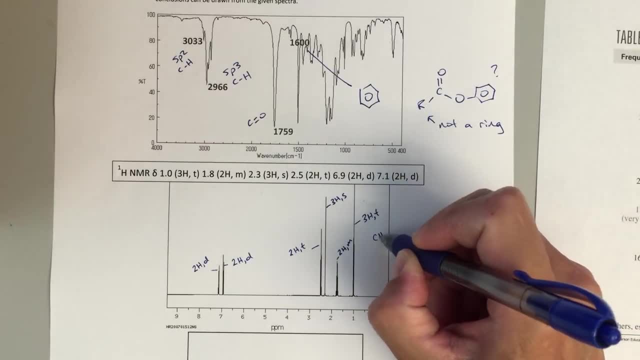 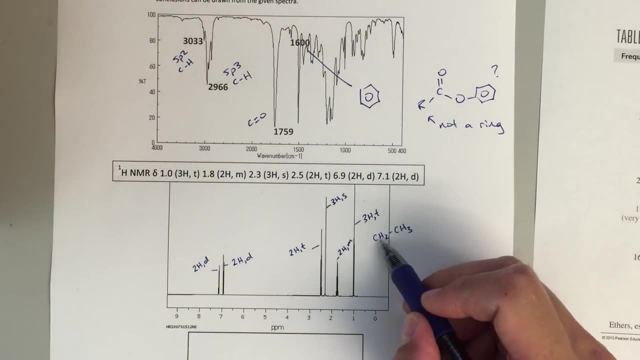 three high triplet. to me, a three high triplet indicates I've got something like this. So this methyl group here that would show up as a three high triplet because it's bonded to this methylene linker, So that would you know, split this methyl group into a three high triplet. This is coming. 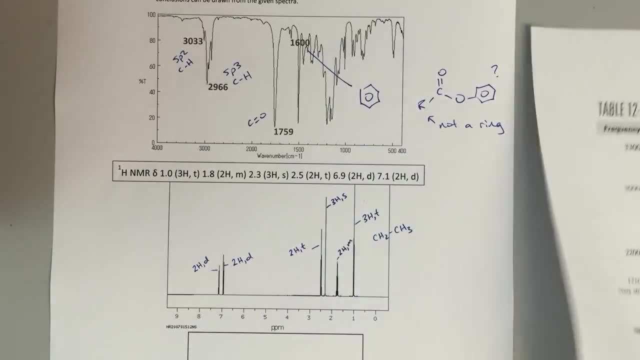 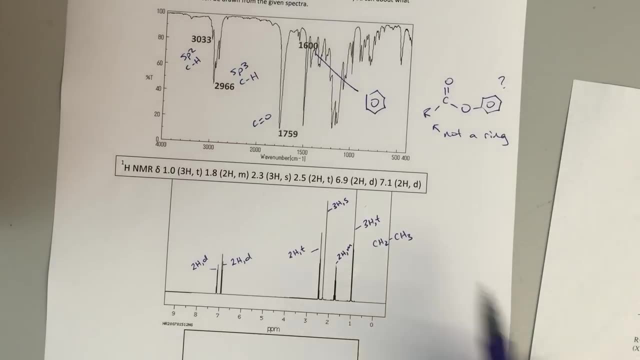 right at about one. So that makes sense for a methyl group. Um, you know, if we, if we turn this table over and we look at where a methyl group is going to come on an alkane 0.9.. So right. 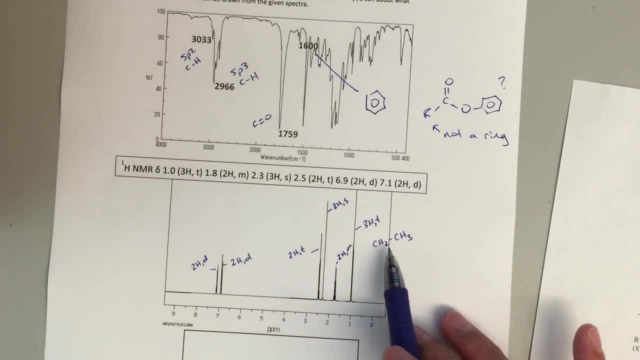 away. this to me says: I've got some sort of ethyl group For this CH2, I think I've got sort of. you know, if this was this say was linked to my carbonyl carbon, then I would expect to see. 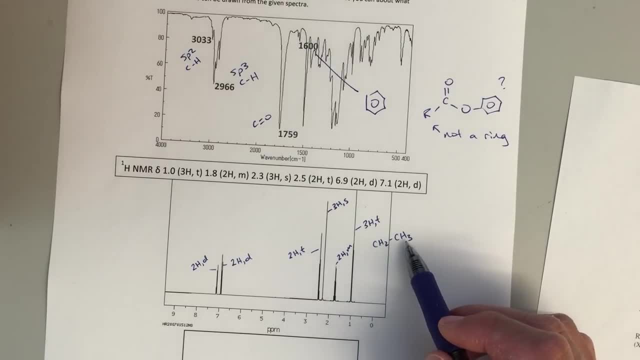 some sort of two high quadruplet, right? Two high quadruplet. I don't see that. but this CH2 is probably linked to something else. And then it's this multiple here, right, Because I've got to have, you know, a two high something. It's not going to be this. two high triplet. 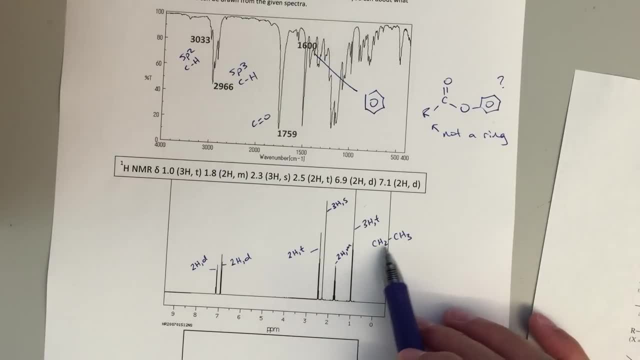 because this would be a quadruplet at least. So this um methylene is probably this peak here, And then that's probably linked to something else. so there's going to be some other CH2 or something else here that I'll have to deal with. 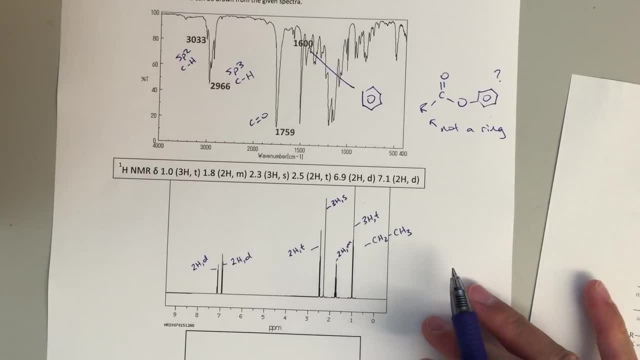 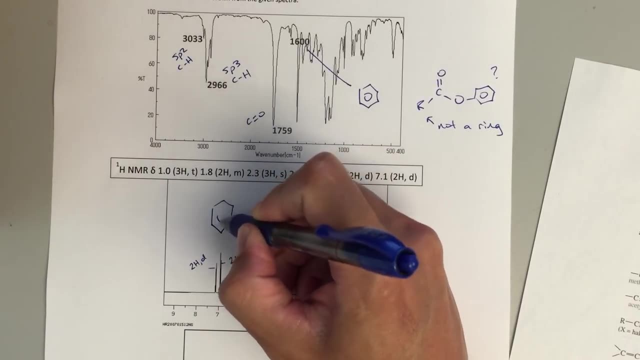 So so far, that's pretty good. The next thing I might say is: well, let's deal with these two peaks out here. These, I think, are very indicative of something. So to me, I'm going to say that these peaks out here. 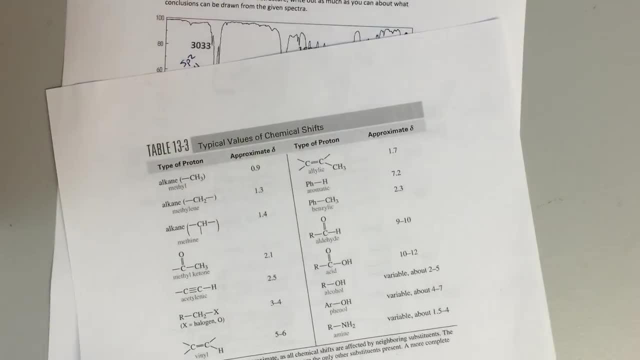 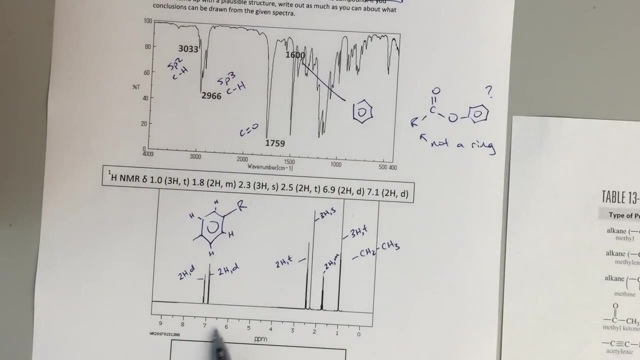 those are probably going to be something on a ring. So if I look at where my phenyl, my aromatic phenyl H, shifts, come approximately 7.2.. We're right here at 7, 6.9, 7.1.. 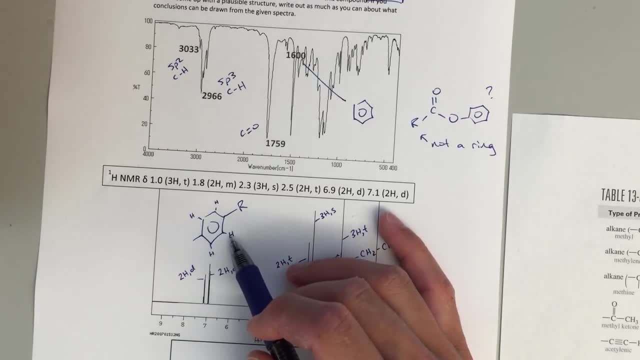 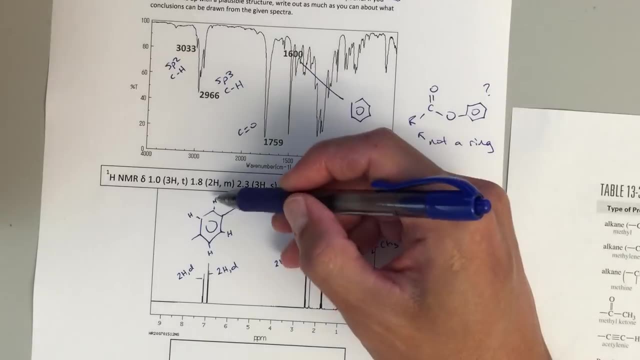 So pretty clearly I think we've got a situation like this I've drawn here where I've got a symmetric phenyl ring, so it's symmetric. I have mirror plane right along here. So two of these: a two-high doublet and a two-high doublet. 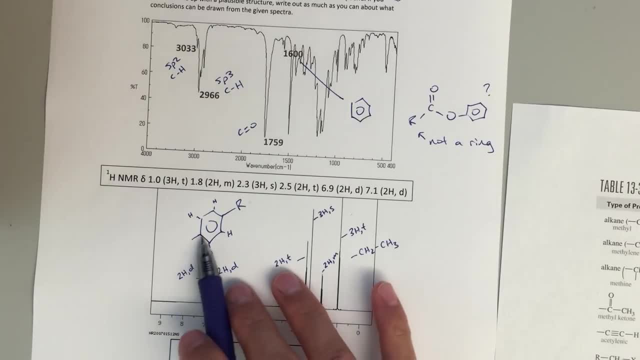 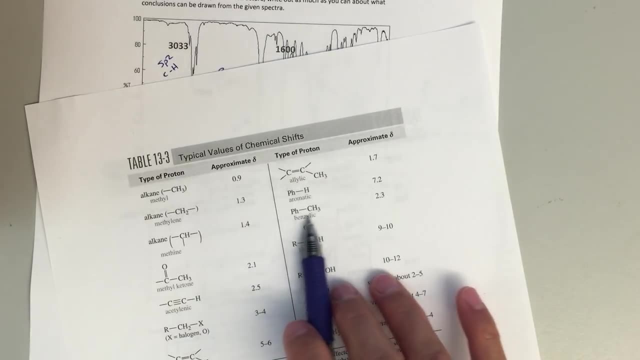 that's what I would expect for something like this. Now, this sort of you know reminds me of this three-high singlet, and that three-high singlet could be a benzylic, a phenylmethyl, so a phenyl with a methyl group on it. 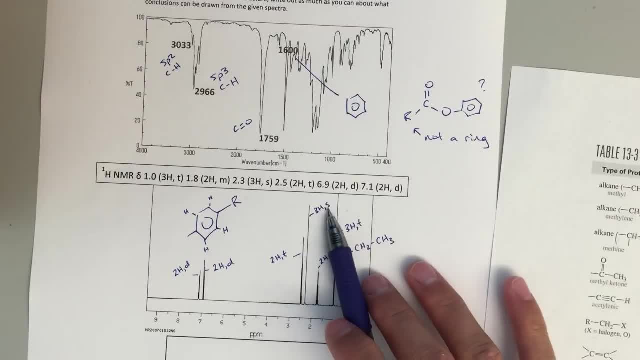 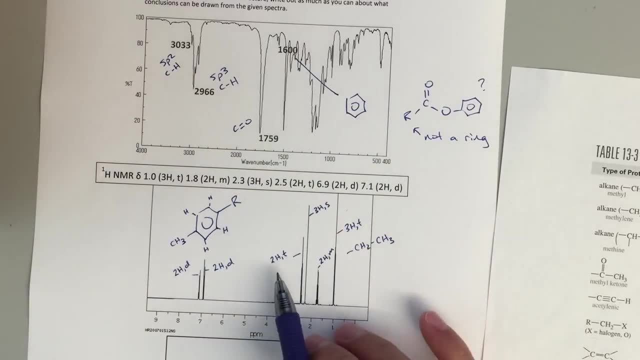 and that comes at approximately 2.3. So my three-high singlet: well, that's exactly at 2.3.. So I'm going to put a methyl group here. I really think that matches up really nicely where I would have an R group coming off here. 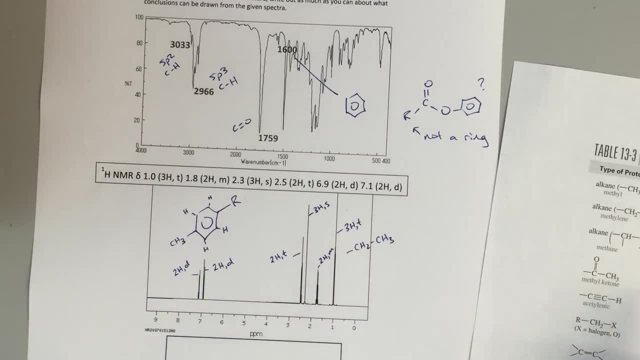 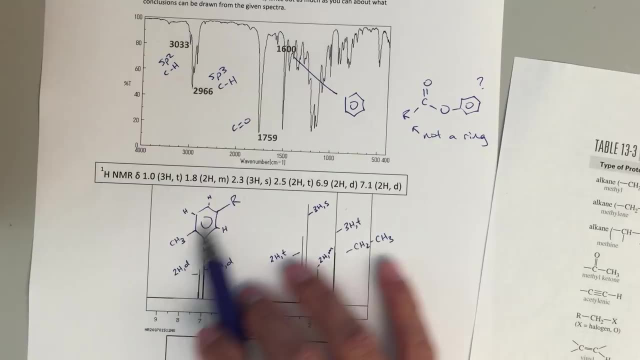 Three-high singlet would be my methyl group on that benzene ring. That matches up really nicely. These, I think, are clearly two-high doublets on that ring. so I've got that mirror plane here. So you know this. I think something like this. 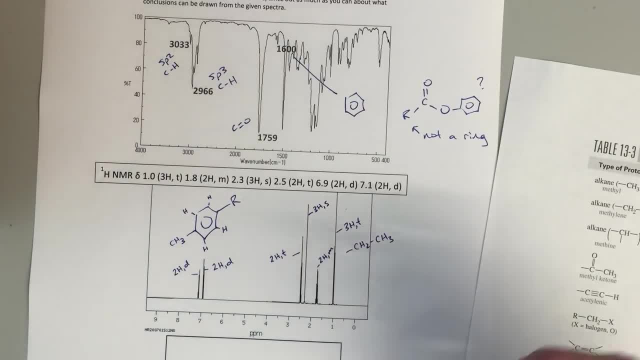 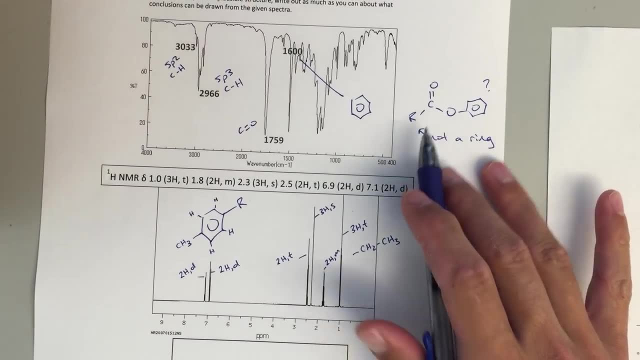 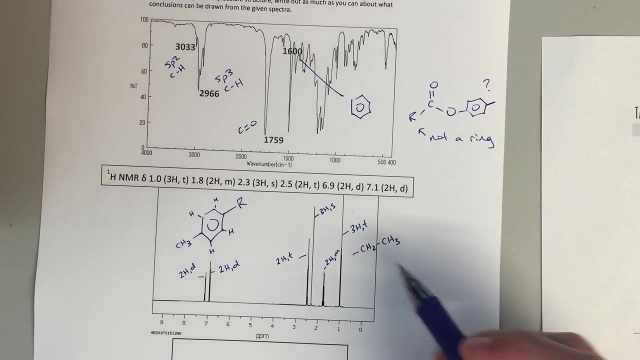 is definitely part of my structure, So let's sort of bring it together a little bit here. We know that we have an ester, We know that we've probably got a ring over here. Now we're going to add that methyl group right over here. 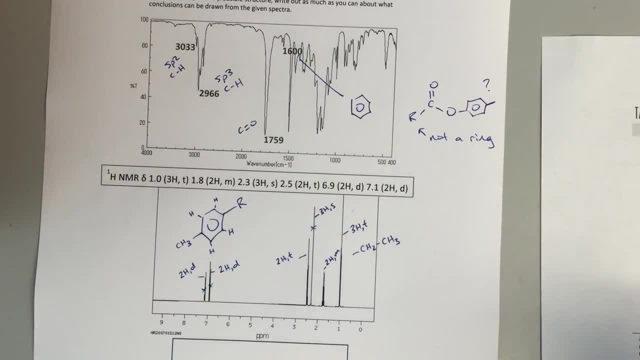 That takes care of this peak, this peak and this peak. I think we earlier said we've got a three-high triplet from this methyl group. This multiplet is probably this methylene, So that leaves this peak over here, a two-high triplet.